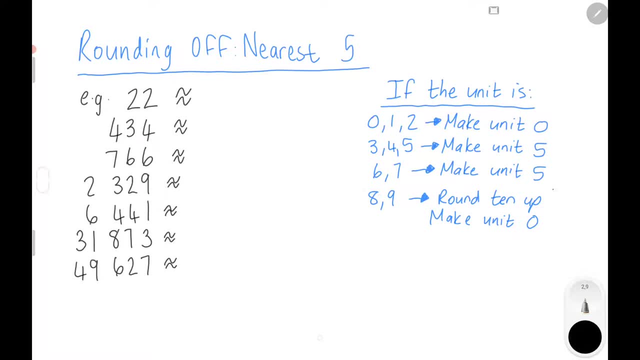 There's only one instance in which you change the 10, and that is this rule around here which we'll look at a little bit later. But otherwise, the entire time we're rounding off to the nearest 5,. it doesn't matter how big the number is. we're only ever looking at the unit portion of the number. 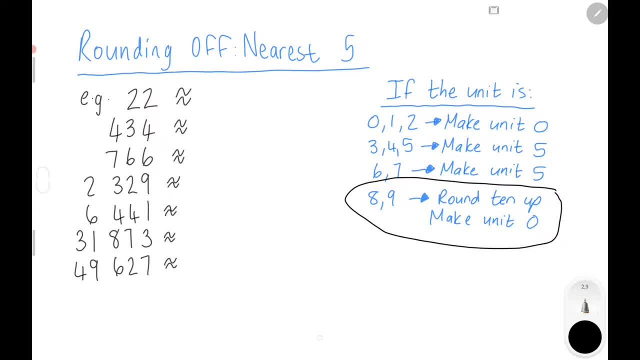 Whether it's a 2-digit number or a 6-digit number, it doesn't really matter. The unit is the one we look at. So let me just take that piece off there. So let's jump right into it. Nothing too fancy. 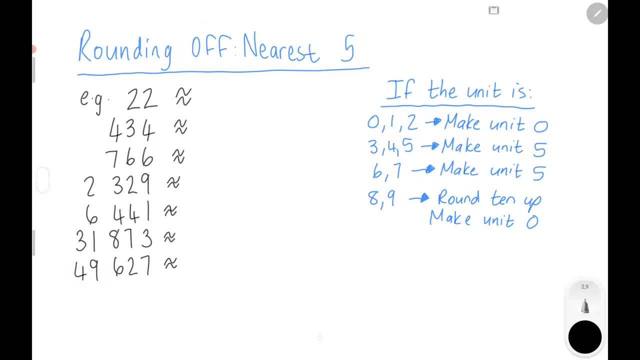 There are four rules, As you all know, with rounding off. there's always some kind of rule that we use to round off. In this case it's not the usual 2 that involve the whole less than 4, more than 5 thing where you round up or down. 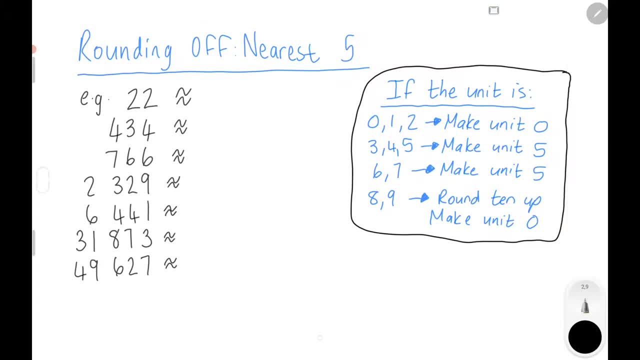 This one actually has four rules, and they are as follows. So you're going to look at the unit and the point is, if the unit is 0,, 1, or 2, then you just simply make the unit 0.. 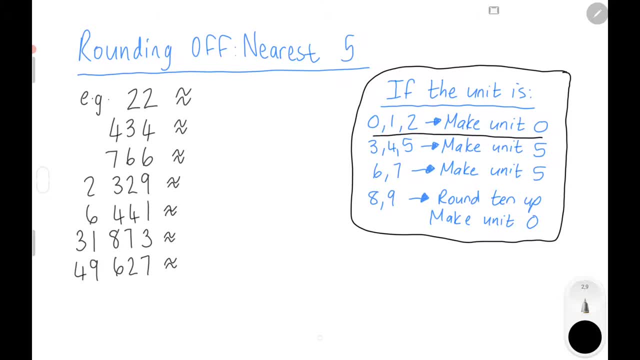 It's easy: if the unit is already 0, you just leave it as a 0.. If the unit is a 1, you make it a 0.. If the unit is a 2, you make it a 0 when you round off. 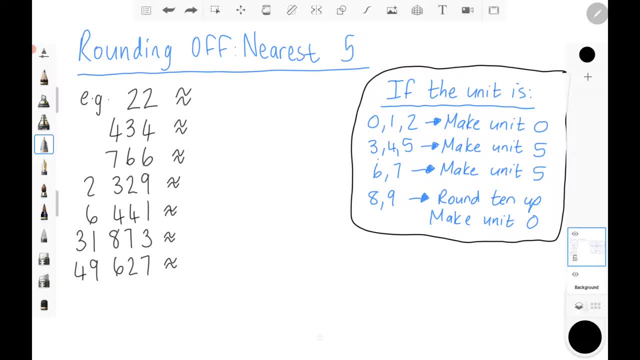 It's as simple as that. Then we have the second rule, which is if the unit is 3,, 4, or 5, then you'll just simply make the unit 5.. So we're rounding it up to the 5 rather than the 10,, that is, below the 5.. 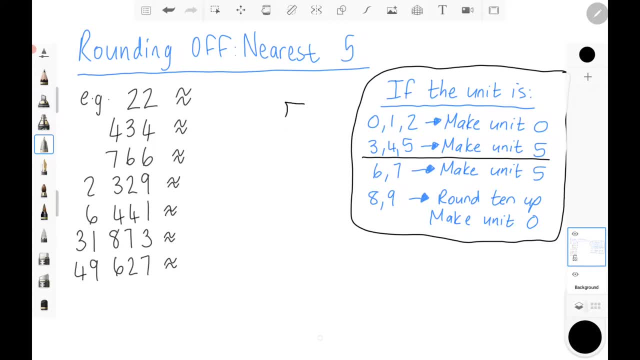 Because we know in the 5 times tables we've got a 5,, then we have a 10.. Then we've got a 5, then we have a 10.. So it's either a 5 or a 10 that we're kind of rounding off to when we're doing nearest 5.. 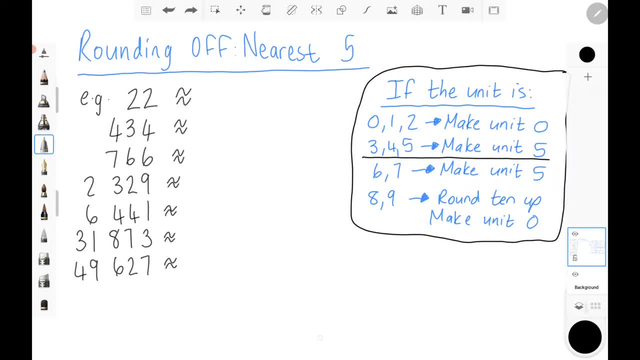 So if the unit is 3,, 4, or 5, you just simply change the unit into a 5.. Then we've got. if the unit is 6 or 7, you'll take the unit down to a 5.. 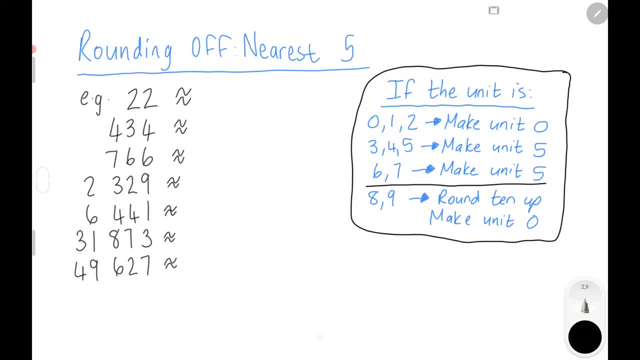 Because we're rounding down 5, or down to the nearest 5,, so we'll just simply change the unit into a 5.. The last one is the more complex of rules, because it's going to involve changing your 10.. If your unit is 8 or 9,, the 10 is now going to go up 1,, as if we are rounding off to the nearest 10.. 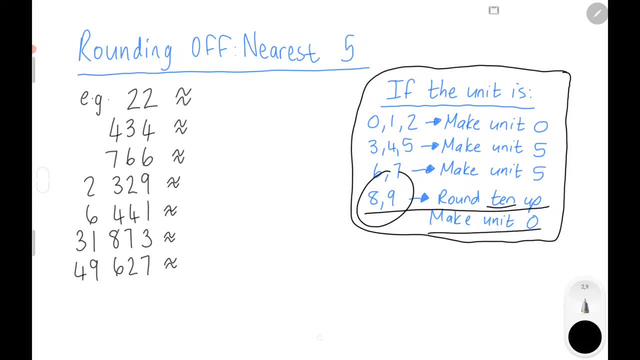 And then you're going to make the unit a 0. So basically, when your unit is 8 or 9, we're actually kind of rounding to the nearest 10. Or rounding up to the nearest 10,, like we usually would when we round off to the nearest 10.. 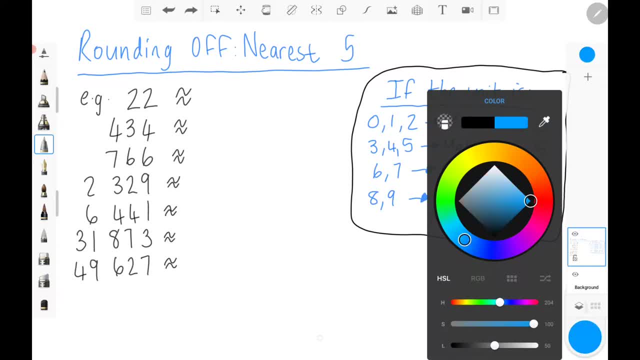 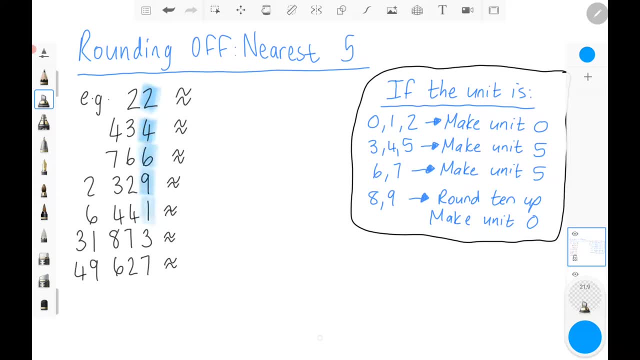 So what I'm going to do is I'm just going to shade our units in each of these practice numbers, Because you should be able to see them. You should always. you know, if you're struggling with rounding off, just take a color pencil and just shade the ones that you're going to need to look at. 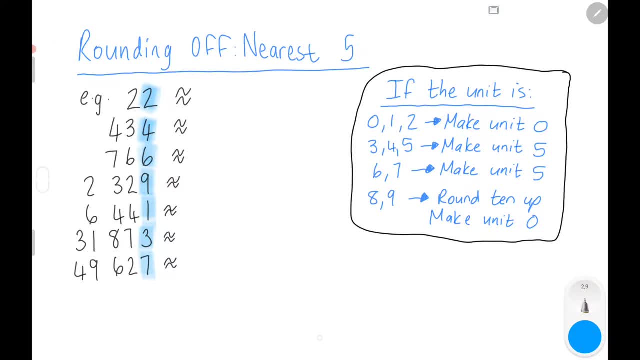 Your helper numbers And then you can do. you know, look at your tens or your hundreds or your thousands, whichever ones. you're rounding off or changing The helper numbers to the right, you're going to need to shade, just to sort of help you out. 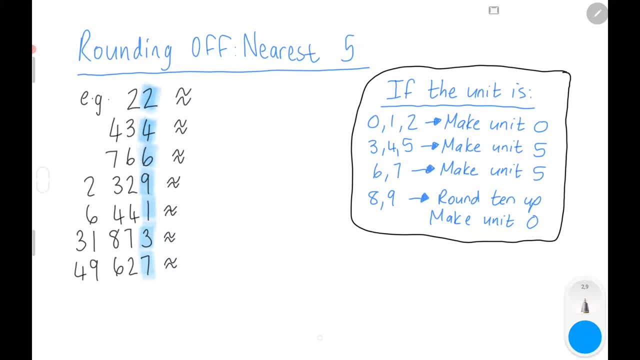 So let's look at these examples. 22 is our first number over here at the top. Now, if we have to round off 22.. Let's look at our rule. What is my unit? My unit is a 2.. So what is the rule if the unit is a 2?? 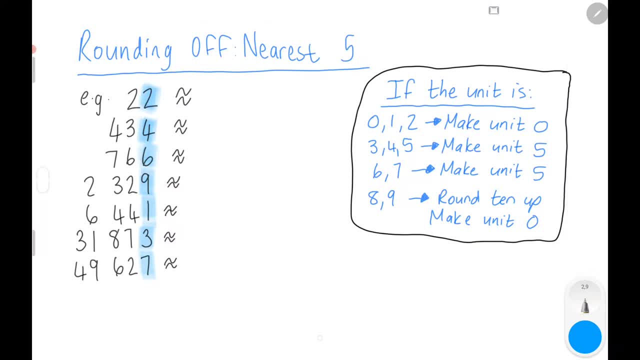 It just says: make the unit a 0. Okay, Which means the unit will be a 0 and my tens stay the same. It says nothing to do with the tens. We don't have to do anything to the tens, Or to hundreds or thousands for that matter. 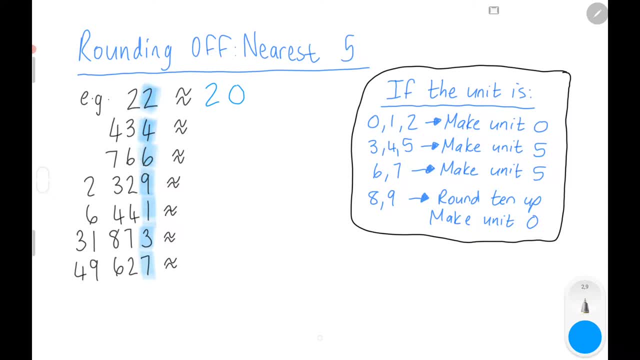 So it just rounds off to 20.. So my nearest 5 is 20.. Let's look at the next one: 434.. My unit is a 4.. And it says: if the unit is a 4. You make the unit 5.. 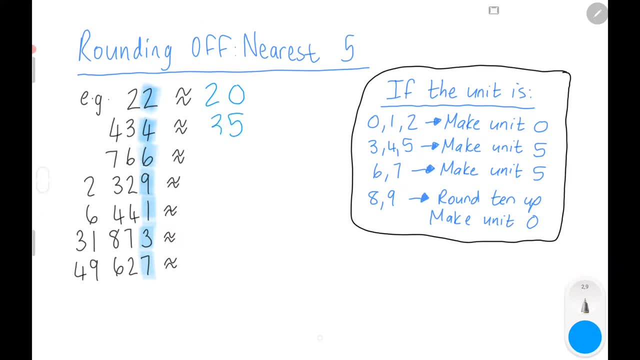 Okay, So my unit will be 5.. The 30 we leave alone, The 400 we leave alone, So 435 is what it rounds off to 766.. My unit is a 6.. And what does it say? You need to make the unit 5.. 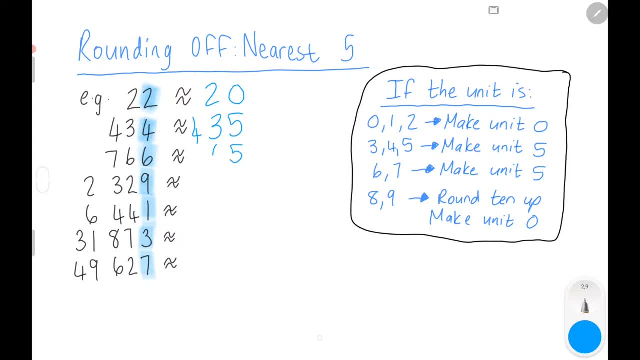 Which means my 6 will turn into a 5.. The 60 stays, The 700 stays And 765 is the rounded off nearest 5.. 2329.. This is where it gets a bit sticky If the unit is a 9.. 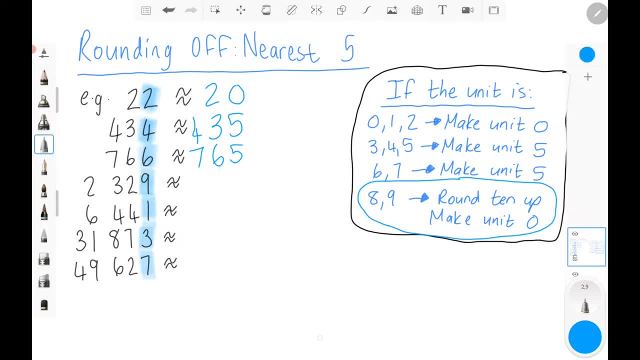 Round the 10 up. Make the unit a 0.. Okay, So We make the unit a 0.. What is the 10?? It's 20, is in our tens place And that needs to go up 1.. So up 1 from 20 is going to be 30.. 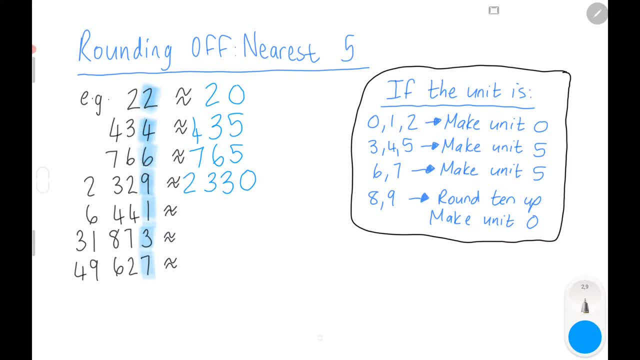 The 300 stays the same, The 2000 stays the same. Okay, So the 20 rounded up to 30. And we made the unit 0.. Alright, Now let's look at the next one, 6441.. What does it say? 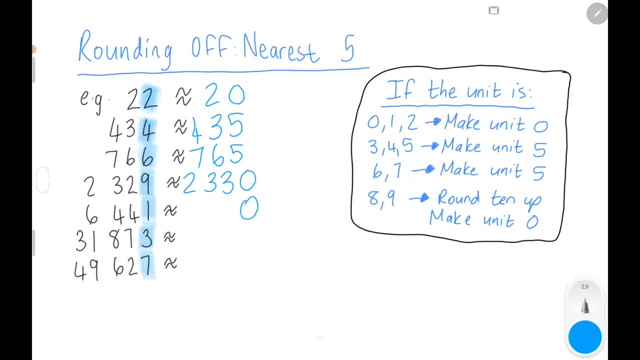 If the unit is a 1.. Make the unit a 0. And you leave everything else as it is- 6440.. Let's look at the next one, 31873.. Maybe you can try this on your own. Think about it. 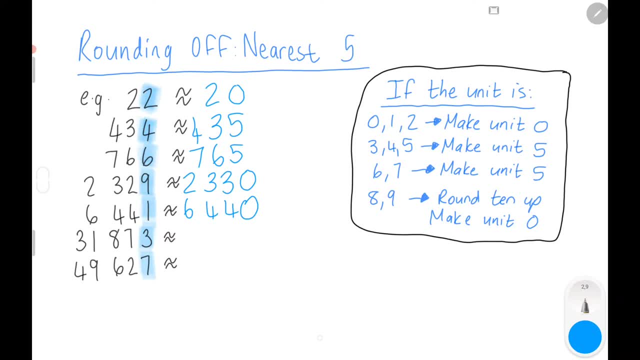 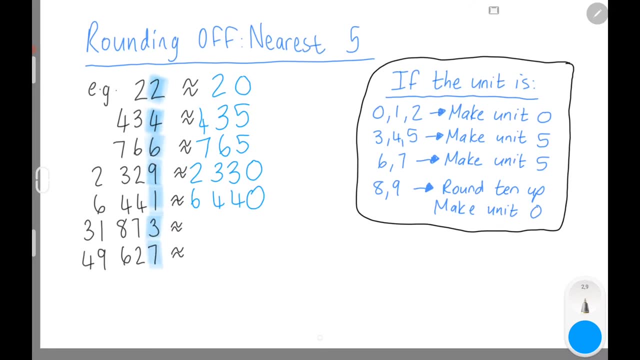 And then I'll answer it for you. If the 3 is in the units column, What do we do? Make the unit? Oops, Let's pull that back. We make the unit a 5.. Then we've got the 70.. 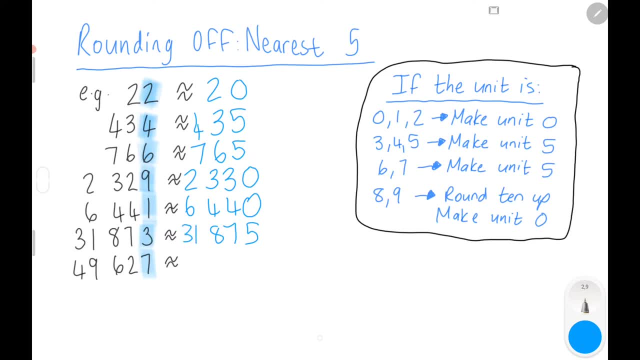 The 800 stays, The 31000 stays. Last one, The unit is a 7.. So what do we do? Make the unit a 5.. 20 stays, 600 stays And 49000 stays, And that is as difficult as it gets. 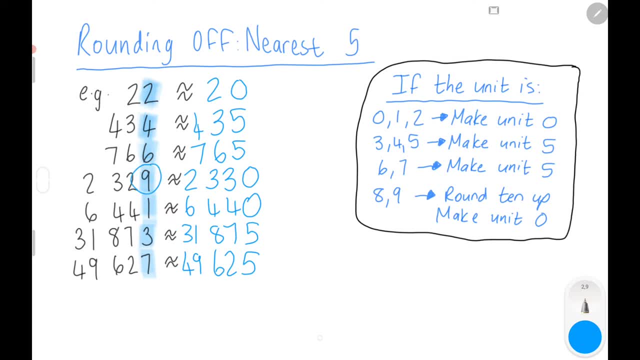 Okay, The only thing you have to worry about are the 9s, Or special cases like, for example, If you were given, Let's say, 26299.. This becomes a problem because Your 9.. In the units column Is going to round the 10 up 1.. 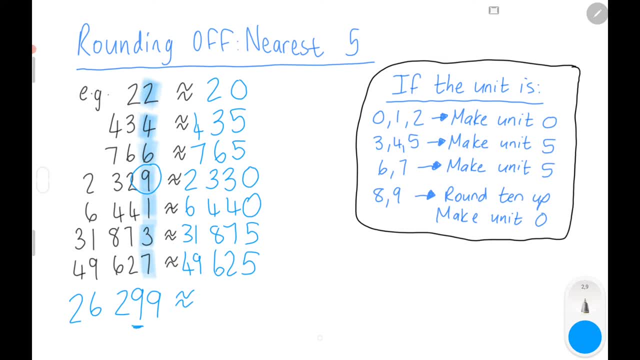 And when you look at the 10., The 10 is a 90. And when 90 rounds up 1., It rounds up to the next 100. Which means your 100 will have to go up 1. Because when the 90 went up,